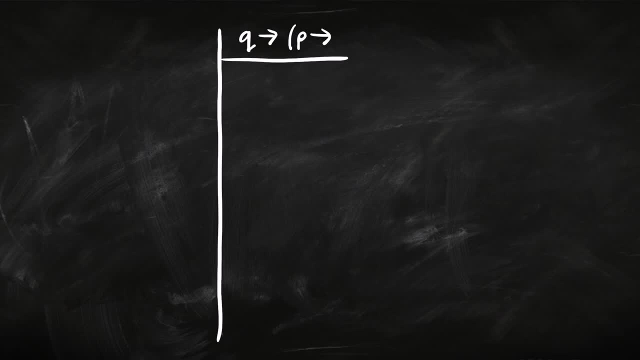 it from this premise. Okay, so we'd write that premise down at the top and this conclusion down at the bottom. and where are we going to go from there? right, We've got something with Q in the antecedent at the top here, but I haven't got Q, so I can't do. modus ponens doesn't like to do. 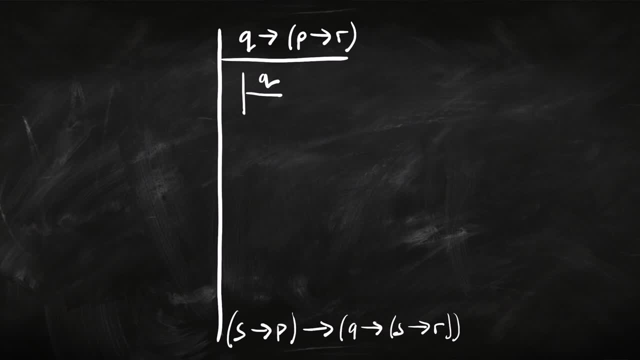 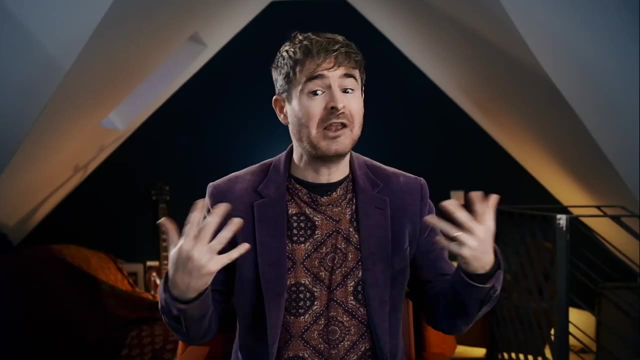 anything else, I might assume Q, because that will allow me to do modus ponens and that allows me to infer: if Q, then P arrow R. but that's what we started with. that doesn't help at all. So we're stuck, we don't know where to go and we kind of get frustrated and give up. And loads of students. 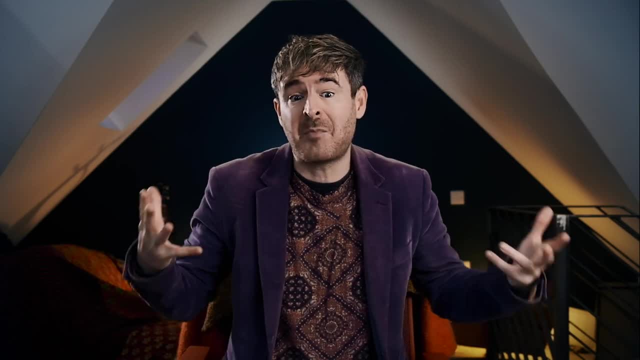 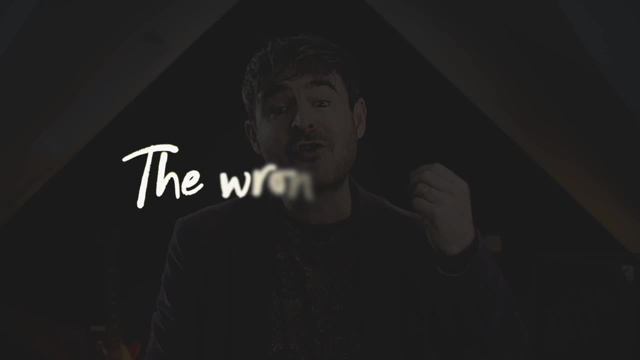 say to me: I just don't get what rule I can apply. next, I don't get how to finish this proof off. Okay, so if that's happening to you, basically what's happening is you've got the wrong strategy. It's not that you don't know the rules well enough or anything like that, you're just going. 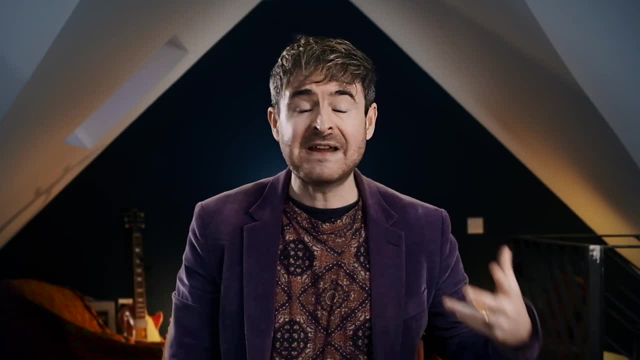 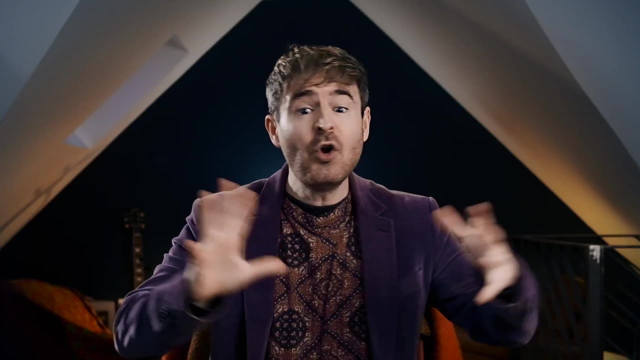 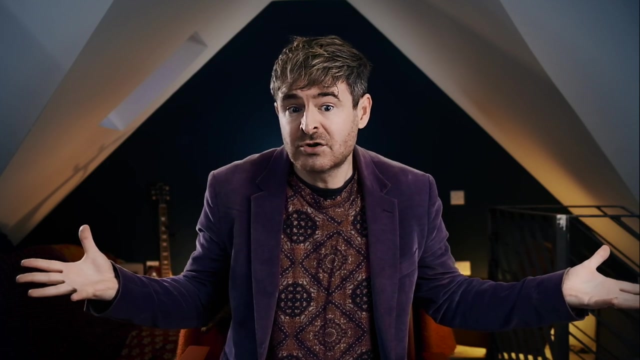 about the proofs in the wrong way. Basically, the reason that this approach doesn't work is that, in natural deduction, we nearly always have to make assumptions, and you're allowed to make any assumption you like. You can assume any sentence. So which sentence should you assume? 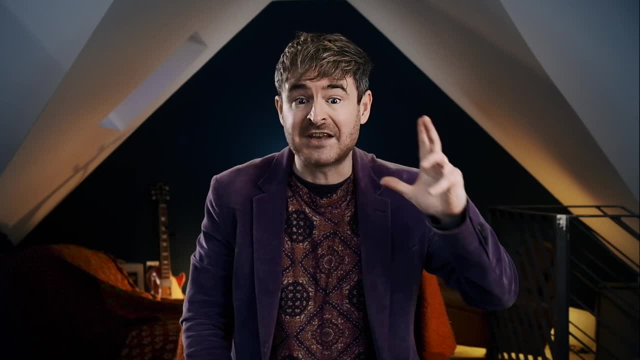 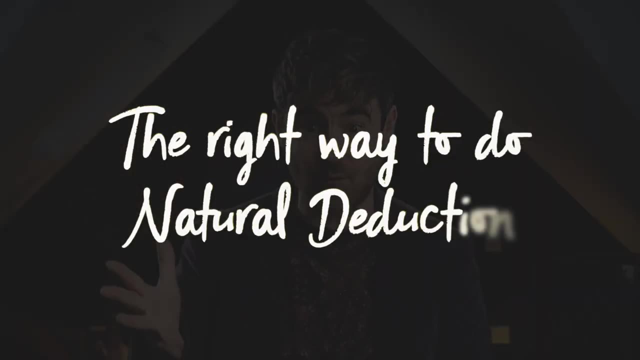 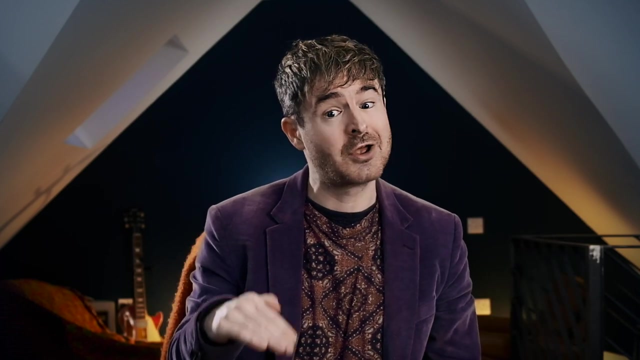 right. It's not obvious. you need some guidance about what assumptions you're going to make. So let me show you. Let me show you how that works. Here's the right way to do natural deduction proofs. So we're given a question. it's got some premises or maybe no premises, but it's always got a conclusion. that's. 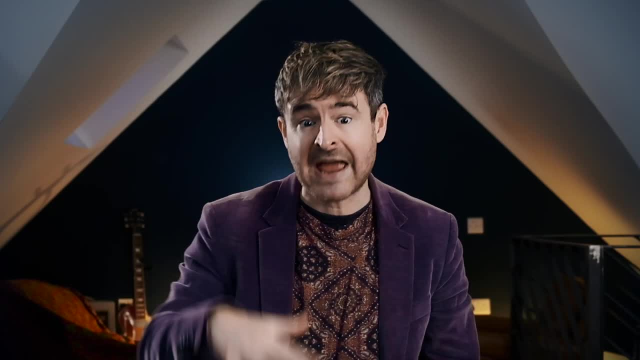 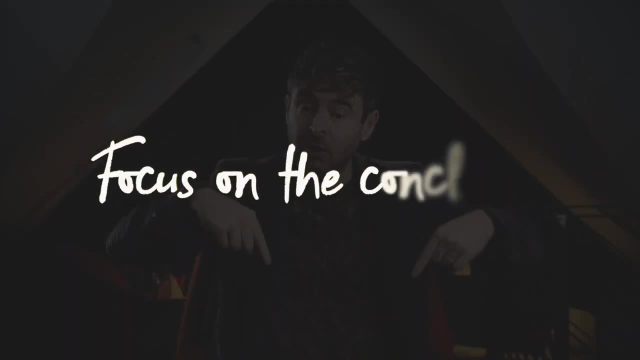 what we're trying to get to. So we're going to write the conclusion down at the bottom of the page and if there's any premises, we're going to write them up at the top. But the important bit to focus on is the conclusion at the bottom of the page. That is our target. that's what we're. 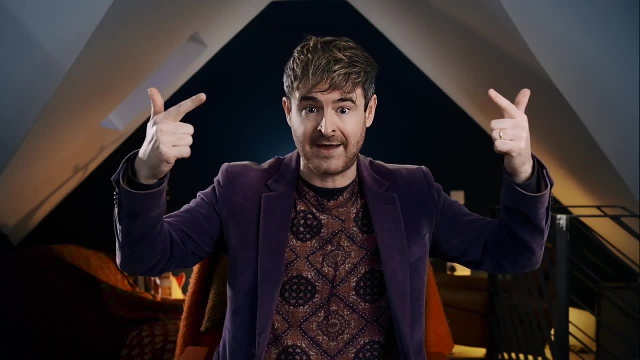 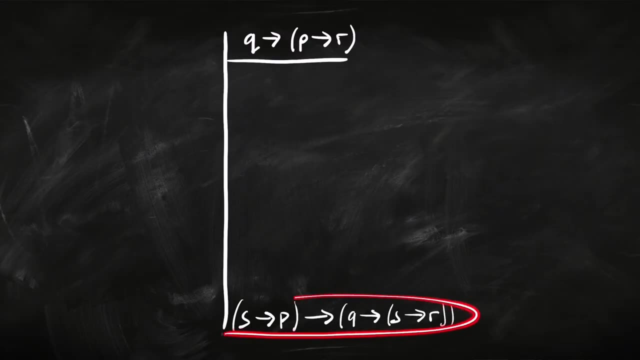 going to look at first and we're going to work up from there. So let's go back to our example and see how this bottom up strategy helps. So we've got this conclusion, this sentence. it's going to be our target and it's an if then sentence: What we're. 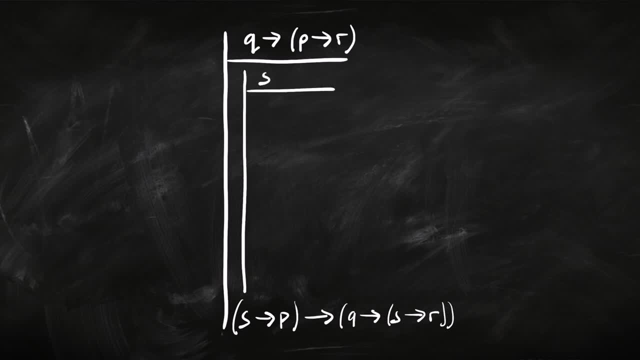 going to do is we're going to assume that antecedent, We're going to assume the if bit, so we're going to write that at the top, the next line down, and we're going to write the then bit, the consequent. 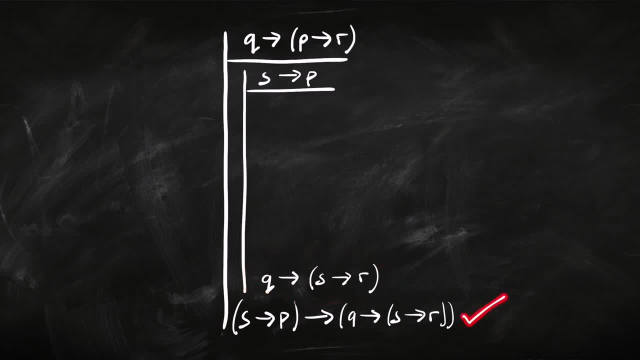 down the bottom, second line up. So we're done with that original target down here at the bottom and the second line up. So we're going to write the then bit, the consequent, down the bottom, second line up. That's going to be our new target. We're going to try and get here, And again it's an if then. 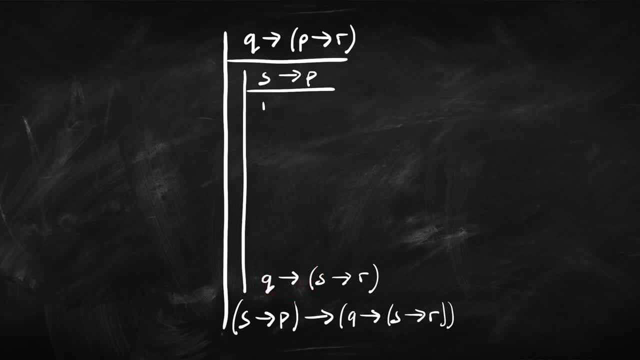 sentence, a conditional. So we're going to do the same thing again. We're going to write Q as an assumption at the top, so third line down now, and we're going to write the then bit: if S, then R. that's going to be the third line up And that is going to be our new target. And guess what? Again? 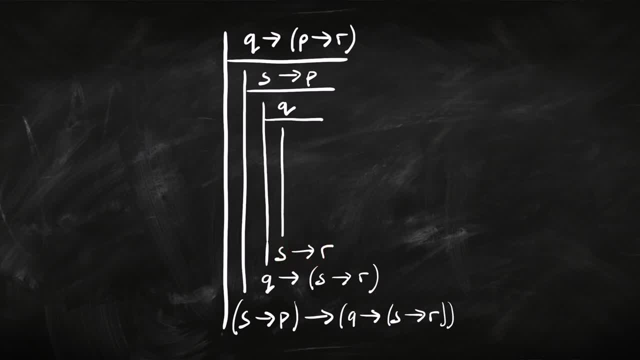 it's an if then. So we're going to do the same thing again. We're going to write the if, the antecedent S as a new assumption, up the top, and we're going to write the then R down the bottom. So that's the fourth line up now. So now, all we've got to do 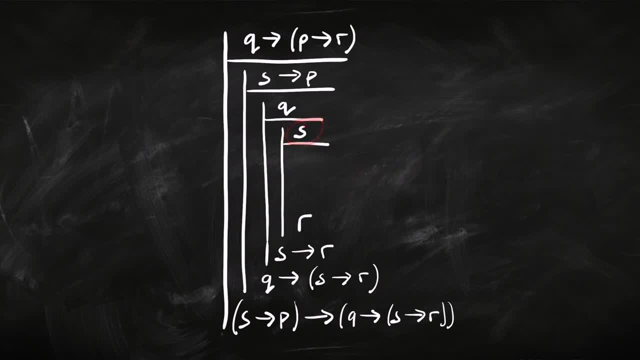 is fill in this little gap between our final assumption S and the conclusion we're trying to get to R Notice how all these subsequent assumptions we've made each is within the scope of the previous. So at this point in the proof we can use all this stuff up at the top here. 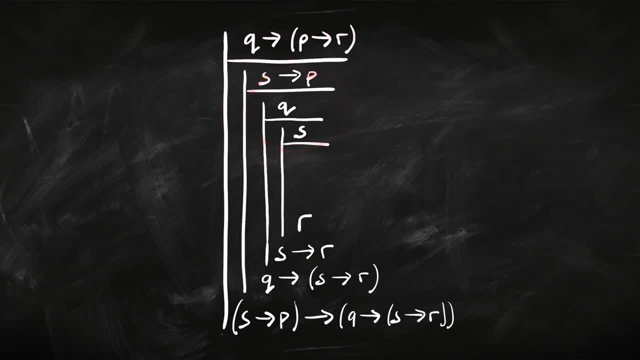 our original premise, plus all the subsequent assumptions. How are we going to get to R? Well, it's not an if, then so the same trick won't work, but still, we're going to take this as our target. We're going to look at all the stuff we've got up at the top and say, how are we going to get R? 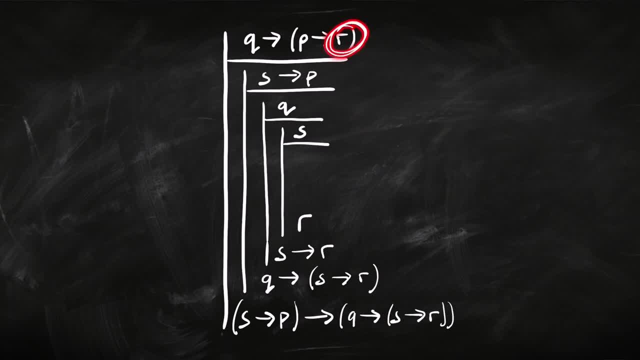 out of them. Well, we've got an R here in our original premise. How are we going to get R out of it? Well, we're going to need to do some modus ponens, so we're going to need to have 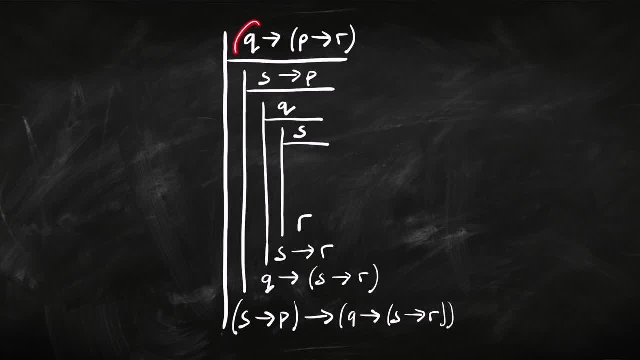 the antecedents of these conditionals. The antecedent here is Q and here I've got a Q as an assumption. so I can infer: if P, then R. And now I'm trying to get this R out of this sentence. How am I going to do that? 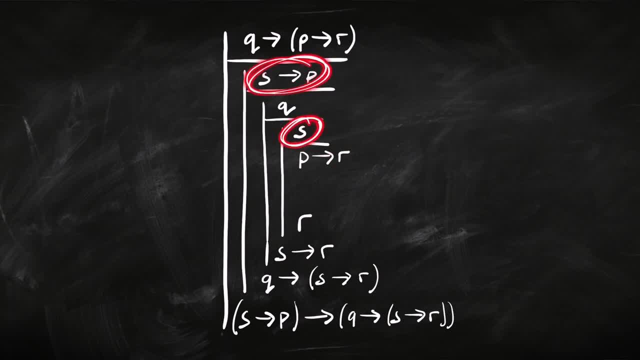 Well, here I've got if S, then P, and here I've got S, so I can add P And combining these two lines, I do modus ponens and I get R out of it. So at that point, this proof.